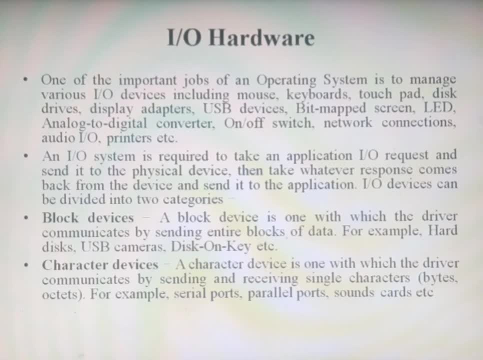 the computer. okay, so these devices will be converting our english language to the binary code and then we will be getting the outputs. so normally what io system will do is it is required to take an application io request and send it to the physical devices, then take whatever response. 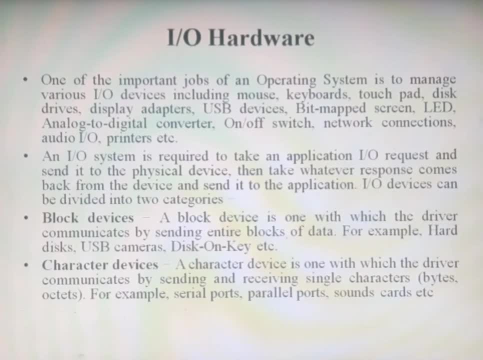 comes back from the device and send it to the application. let's suppose i have given an input like 2 plus 3 by using a keyboard. i have used an interface called keyboard and i have given my input. that what is the result of 2 plus 3? i entered 2 number plus symbol. 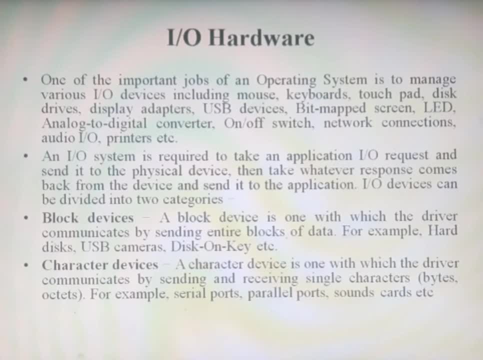 and 3 number. so now that has to given give the output. and whatever the output is given, that is called a response and that response will come back from the device. so now let's say i have given an input like 2 plus 3 by using a keyboard. 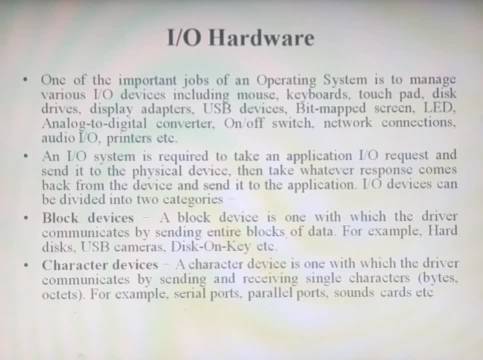 and that will be given to the application. whatever the application you are using, okay, let us say that if you are using a calculator, okay, and that is one of the application in that calculator, you pressed 2 plus 3, okay, and that 2 plus 3 will be converted into the binary code. 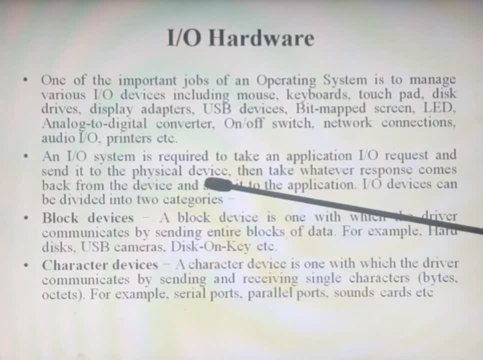 and through physical device you are giving that input. okay, that physical device is keyboard. now i am using keyboard. okay, through physical device you are giving an input and here that 2 plus 3 will be converted into the binary code and a response will come and whatever. 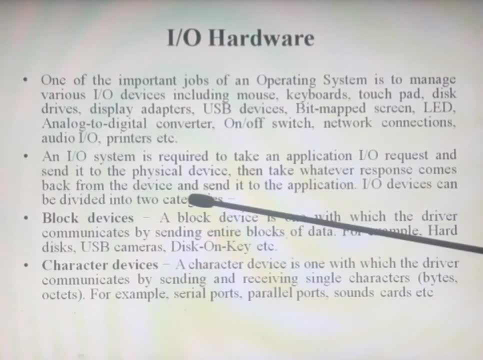 the response comes back from the device that will be sent to your application, called calculator. okay, this is how communication will be done. okay, so there are two types and two categories will be there for this: sending and receiving the inputs. those are block devices and character devices. we will see them one by one. 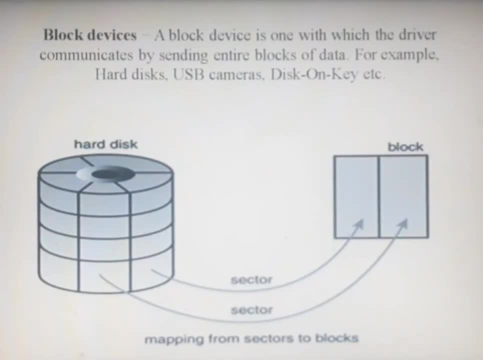 okay, the first one is block devices. okay, a block device is one of one with which driver communicates by sending entire blocks of data. so all at once, so hard. let us take the example of hard disk. this can be a hard disk, usb, cameras, disk on key, etc. 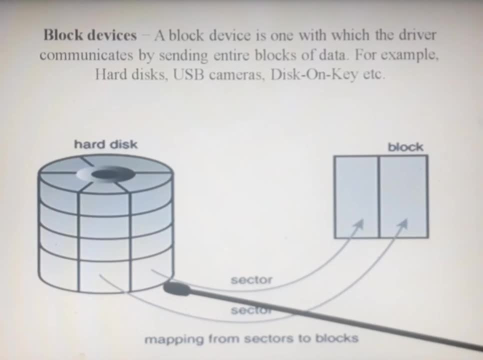 okay, let us take the example of hard disk here. so this is the hard disk and this is the main memory, okay, so, as i told you, in secondary memory each and every block is called as pages and in the main memory they are called as frames. here also, there are 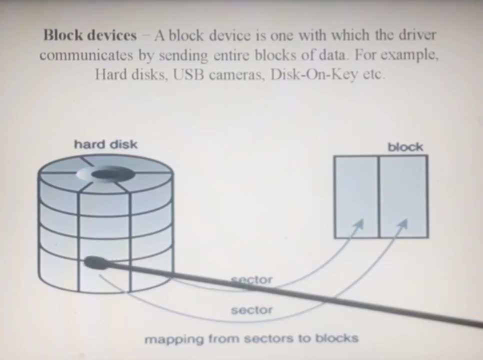 two names. see a hard disk in. in hard disk, this block is called as sector and in main memory, this block is called as block. okay, so in block devices, what happens? complete set of data will be transferred to the main memory. okay, this complete block, okay, this total sector will be transferred to the block. 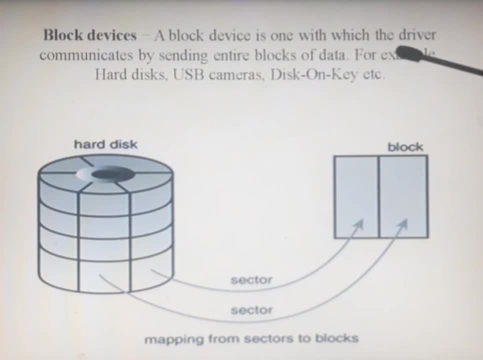 okay, so a block device is the one with which the driver communicates by sending entire blocks of data. you can communicate with any of the device, not only hard disk. you can be communicating with the cameras disks, anything but here what happens? entire block of data will be sent to the memory. 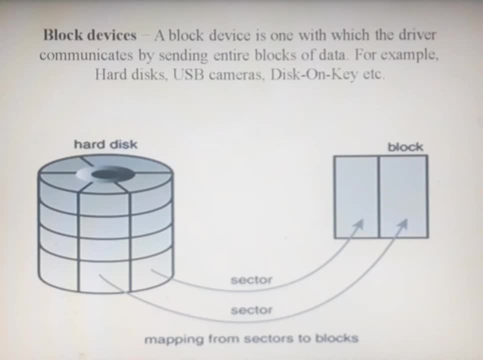 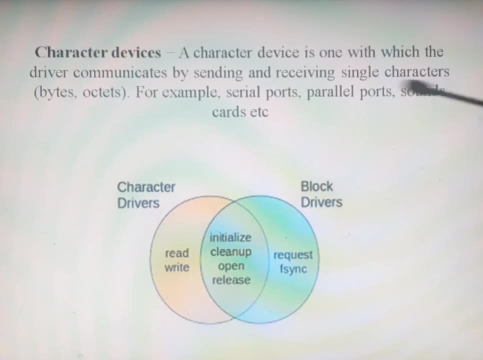 okay, that is nothing but block devices. the second one is character devices. this is a second one. in character devices, what happens? it is the one with which the wire driver communicates by sending and receiving single characters, only only single character, like bytes or text, like that. okay, for example, this will be: 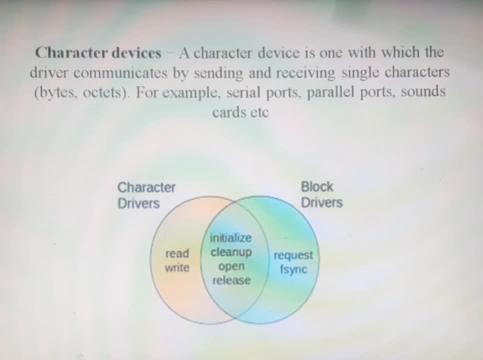 done by using serial ports, parallel ports, sound cards, etc. if complete block of data is going to be transferred, then we use block devices. if only bytes and octets are need to be transferred, then we use serial ports, parallel ports, sound etc. you may ask me, like y, how we will be giving input as one character like that. see in the first example we have. 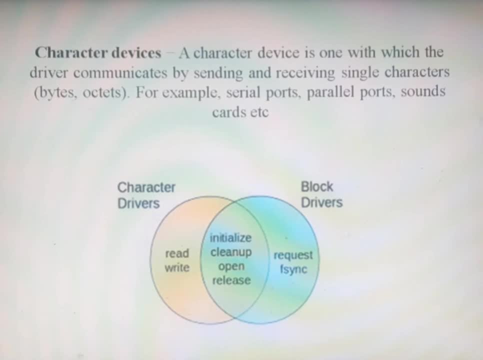 seen you have entered two and three. those are single characters. when you're entering, i mean when you are giving input a single character, then you that uses character devices. but if you are connecting some hard disk to your computer and you want it to transfer file, that is taken care by the